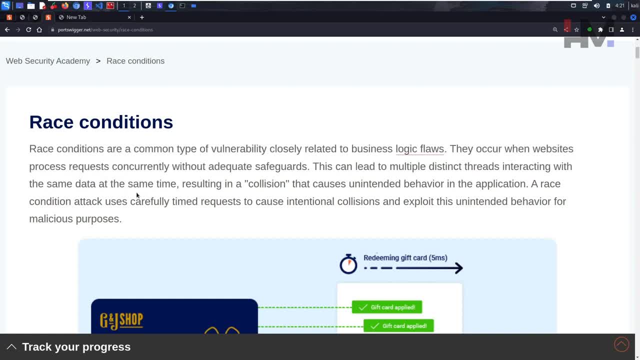 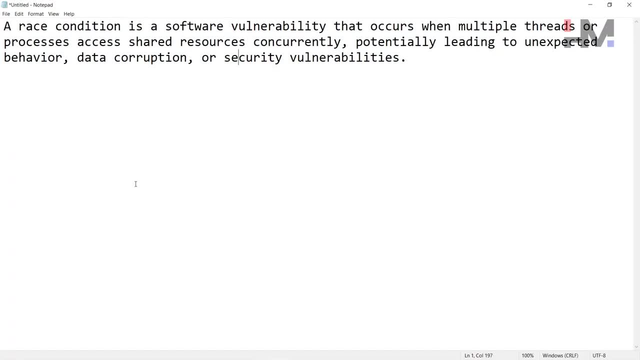 but this is not a particular definition. Okay So, let's see the definition first, and then we'll continue with this. Okay So, this is how I want to define race condition. Okay So, a race condition is a softer vulnerability that occurs when multiple threads or processes. 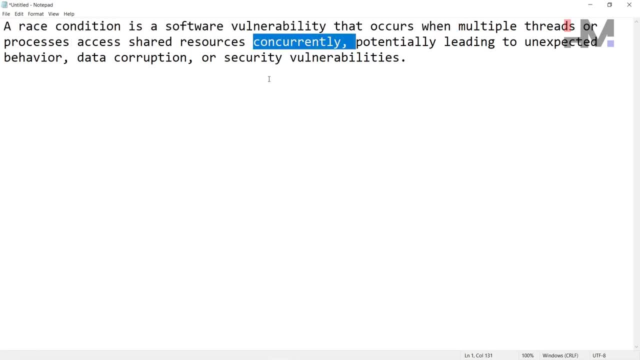 access shared resources concurrently, which means, at the same time, multiple threads and multiple process want to access the shared resources at the same time. Okay, So that's what it means And what it does is it potentially leads to unexpected behavior, data corruption. 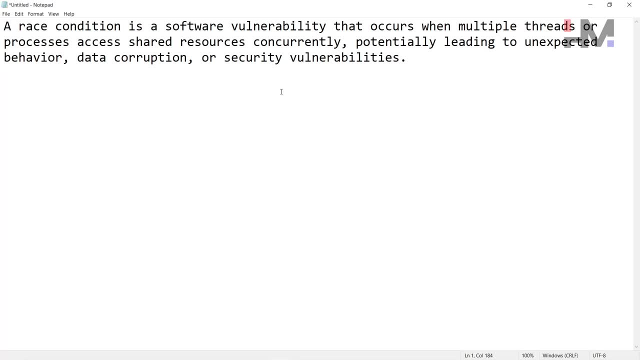 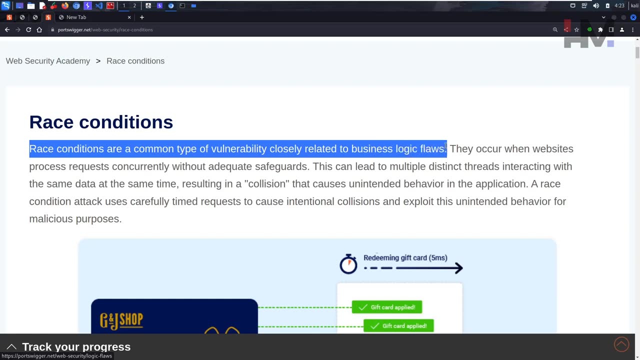 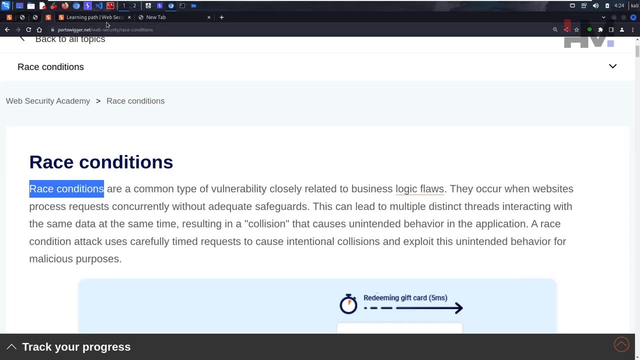 and security vulnerability. Please let's jump into the port sugar labs. So what do we have here? Okay, Race conditions are common type of vulnerability closely related to business logic flaws. Okay, So what they are trying to say is: so race conditions are a subtopic of this business logic flaws- Okay. 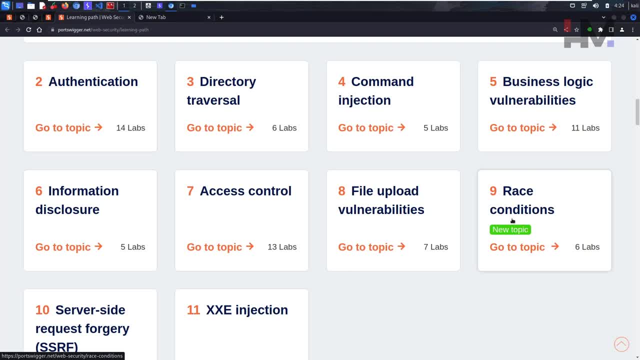 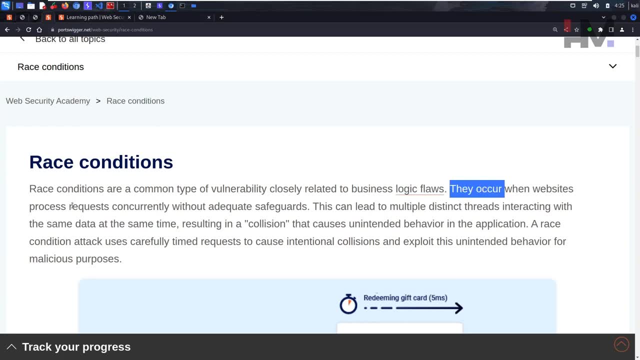 These days, race conditions have become so much important that they needed their own space. Okay, Let's continue. So the first condition is that website process requests concurrently without adequate safeguards. Okay, So this is why it is happening. Okay, So these are all just. uh, these can lead. 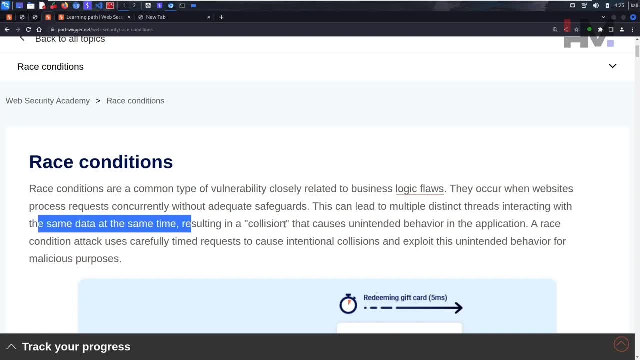 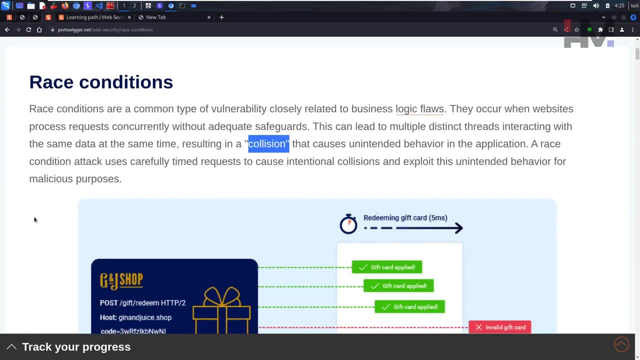 to multiple distinct threads interacting the same data at the same time, resulting a collision that causes unintended behavior. by collision They mean, uh, they're occurring at the same time. A race condition attack: uses carefully timed requests: Okay, So this race condition is totally dependent on time. Okay, So, uses when carefully timed. 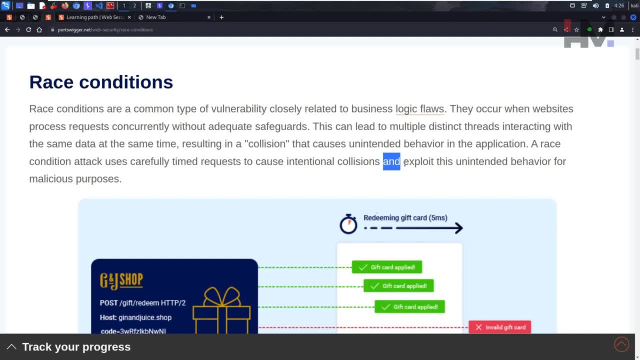 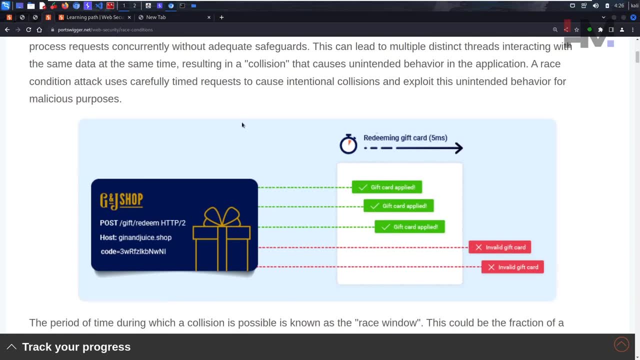 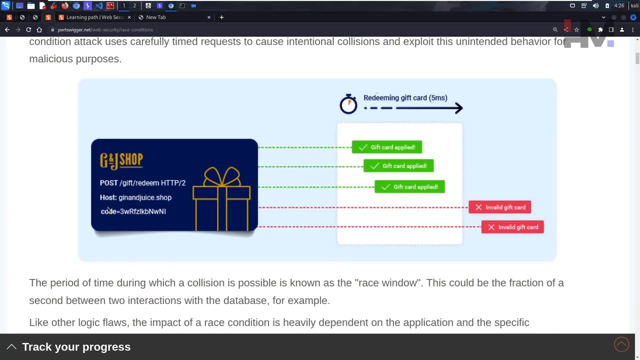 request to cause intentional collisions and exploit this unintended behavior for malicious purposes. Okay, So they have given an example, using an image So, in which they are saying that they want to redeem this gift shop. Okay, So, instead of sending one request, they're. 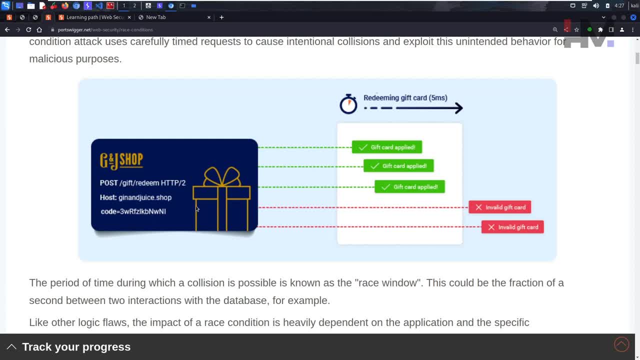 They just make a copy of this request a hundred times or so, in this case five times. okay, They want to send all the requests at the same time. All these five requests has to go through the server at the same time. but here they. 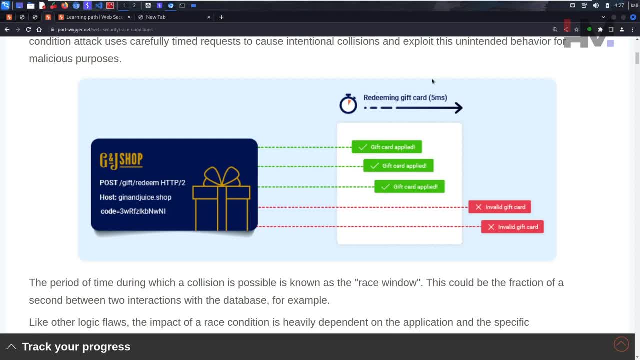 have shown some variation in time. Okay, So what happened is these three requests have been applied. So what they are saying is: this single gift card is equivalent to three gift cards. So that's what they're saying. So if you try to use a multiple request within this five milliseconds gap, okay, 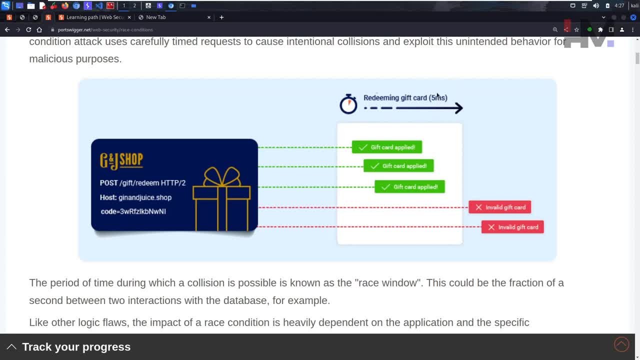 So this is just an example. okay, Five millisecond is an example, but anyhow. so if it is able to get within this five millisecond, depending on how many requests that go through this five millisecond gap, those are being redeemed. 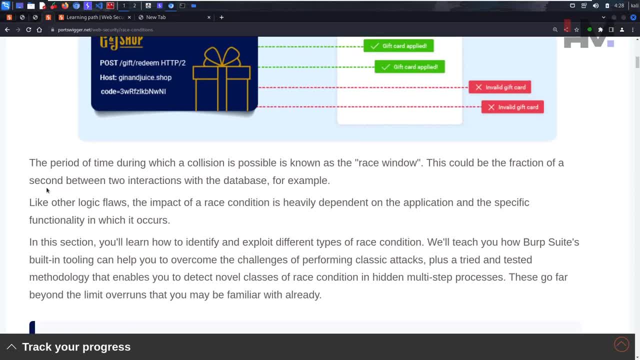 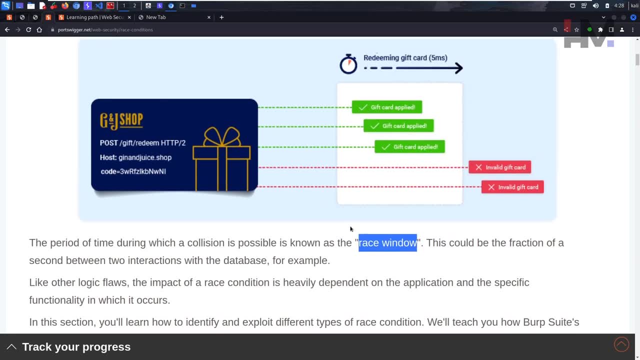 Okay, Let's see. So the period of time in which a collision is possible is known as a race window. Okay, So this period, whichever is there, is called a race window. Okay, So this is the period. This is the time. 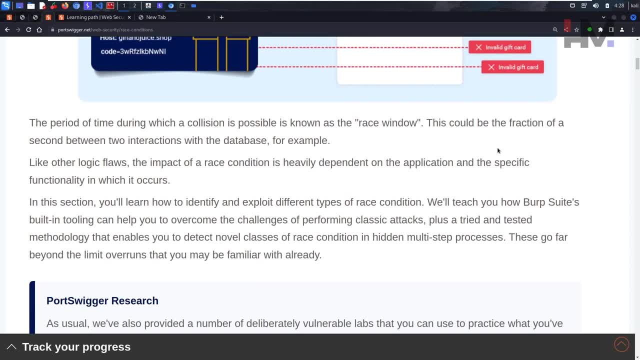 This is not just a window. Okay, This is a time, So this could be fraction of a second between two interactions with the database, for example. So next line they're saying that has heavy. Okay, This is really dependent on application specific functionality. 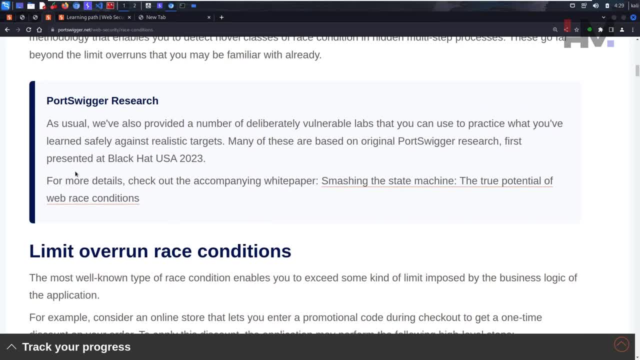 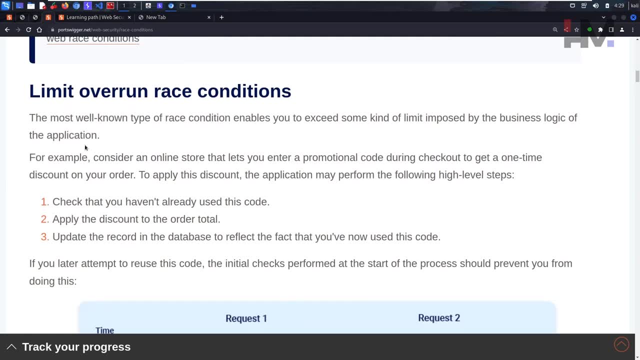 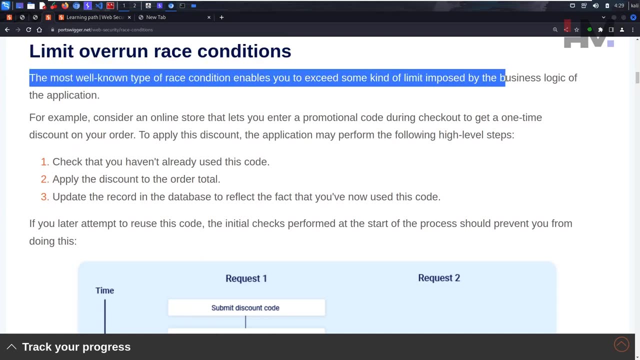 So this was first presented in black hat, USA 2023.. So this is very recent, Okay. And let's see, we have limit overrun race conditions. Okay, So the most well-known type of race condition enables you to exceed some kind of limit imposed. 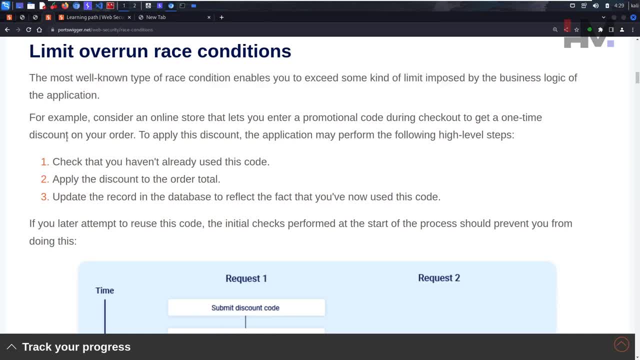 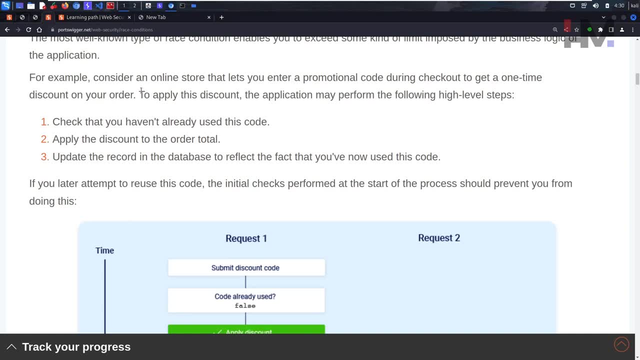 by business logic of application. So here they have an example in which they want To apply a promotional code, or a promo code Okay. So while applying this promotional code, okay, what are the things that usually happen? first, you check the promotional code that you haven't used it. 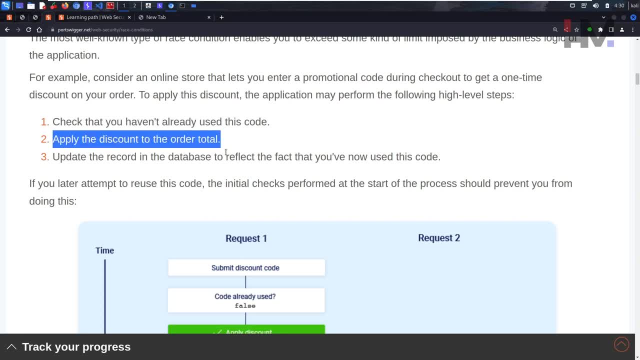 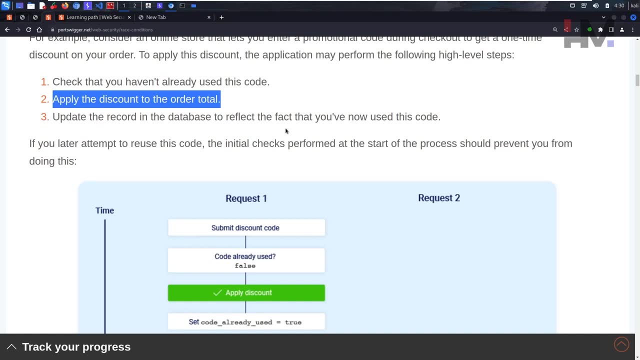 Okay, And secondly, apply the discount code to order total: Okay. So, after applying the coupon code, what is the remaining amount that we need to pay? Okay, So that's the thing, And it will update the record in the database. 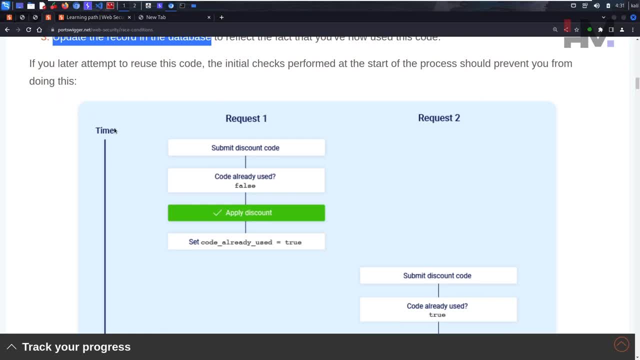 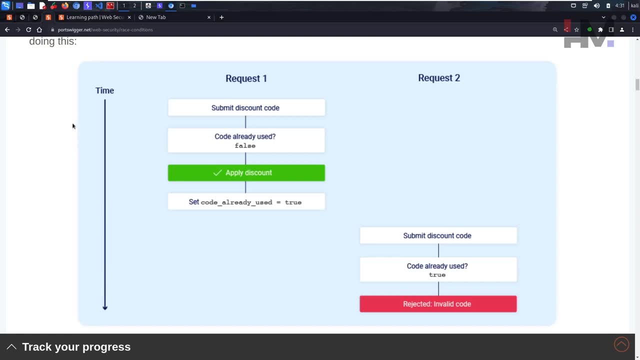 Okay, So these three things happen and let's see. So this is the time that usually happens. Okay, So when we try to use the code for the first time, what happens is it will simply apply the discount. Okay, So the next time we try to use the same promo code, this is going to happen. 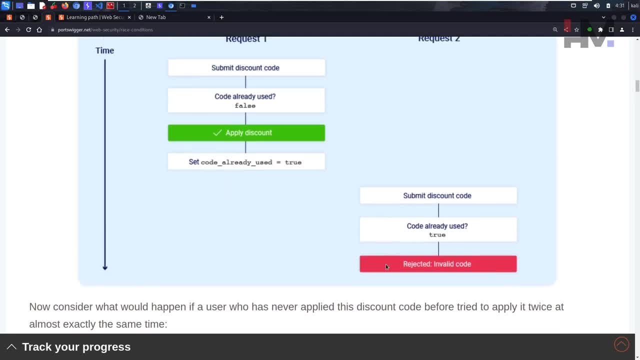 Okay, This will be rejected. Okay, So what they're trying to say using this time is: so this: you have already applied once this. you wanted to apply for second time. Okay, Which is not going to happen. Okay, All of this we will see practically in a web application lab. 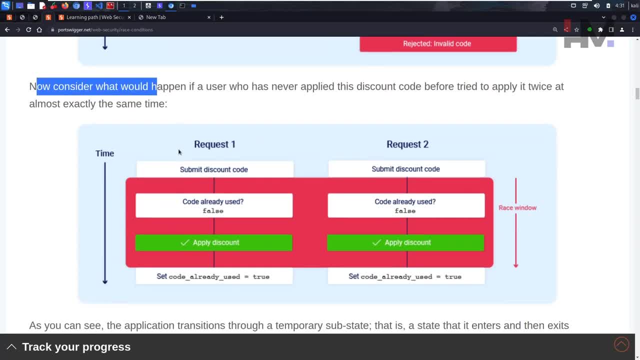 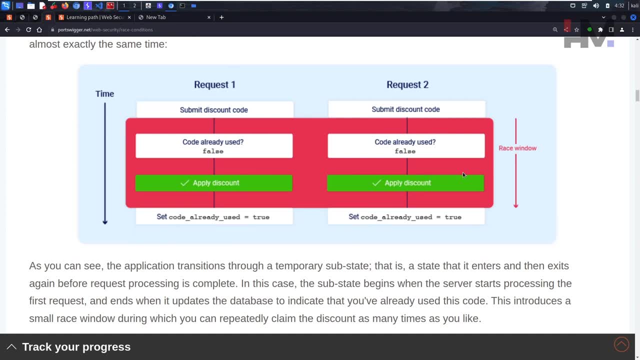 Okay. So what will happen if you send these two requests at the same time? if the code is being checked in the same race window, Okay, Then both of these codes will say that code is not used. Okay, Code already used false. code already used false. 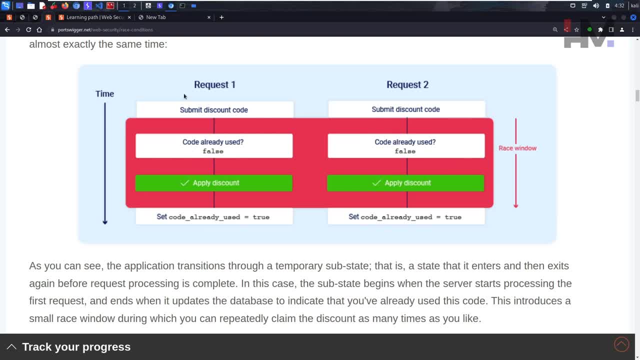 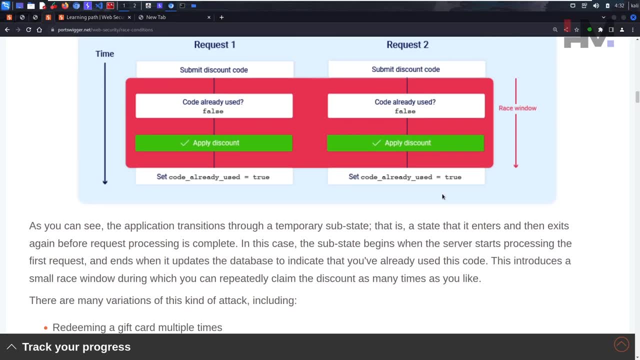 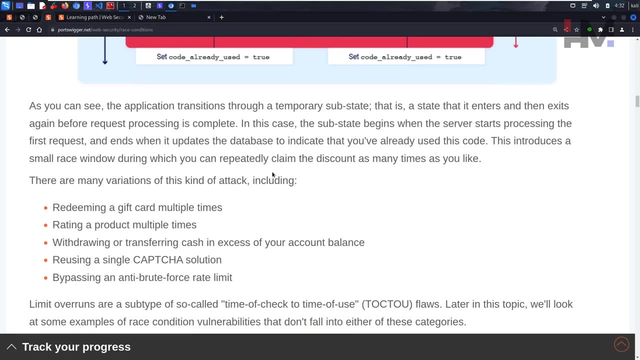 So in this small period of time when both the requests reach the server, then both the codes are being applied. The remaining amount that we need to pay is even lesser than the previous one we discussed here. Okay, So that's how it is. 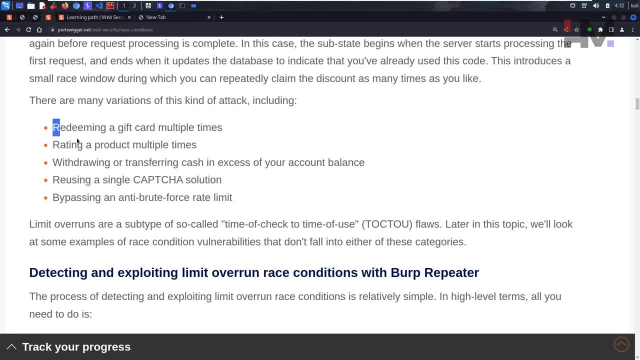 So where can you attack? Okay, Okay. So there are two situations where you can attack it: Okay, Bypassing anti-brute force race limit. Okay, Redeeming a gift card multiple times, rating a product multiple times, withdrawing or transferring. 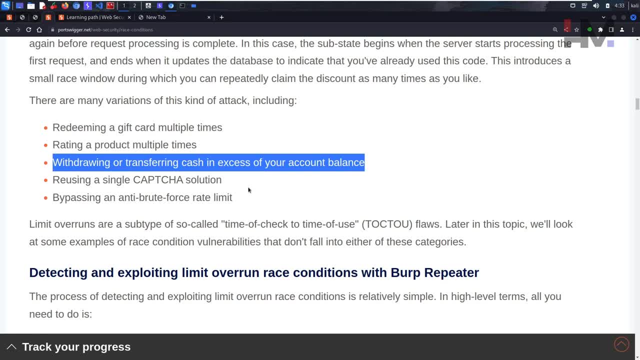 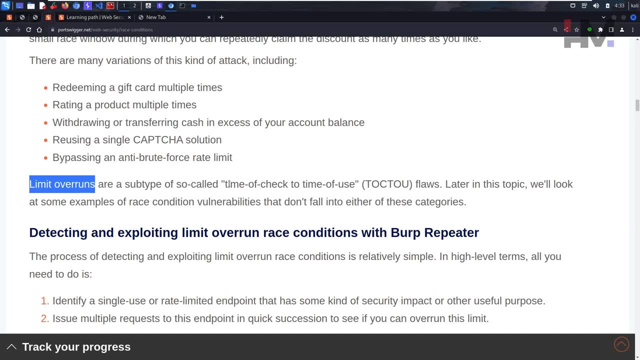 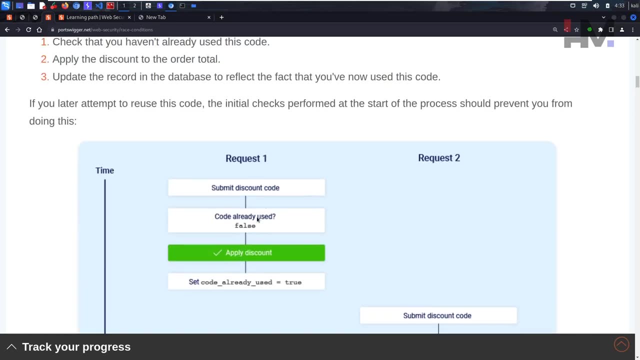 cash in excess of your bank account Interesting. So limit overruns. Okay, So these are just a subtype called time of check to time of use. So this you can understand using this example. Okay, So this is the time of check. 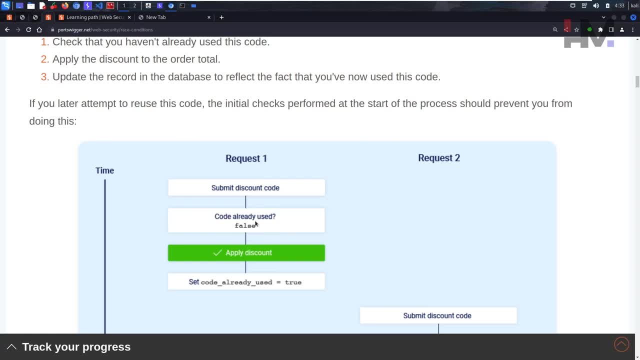 Okay, So this is actually checking this time and this is the time of use code used already. Okay, So this is the time of check and time of use. So these are called limit overruns. Okay, So let's see a lab. 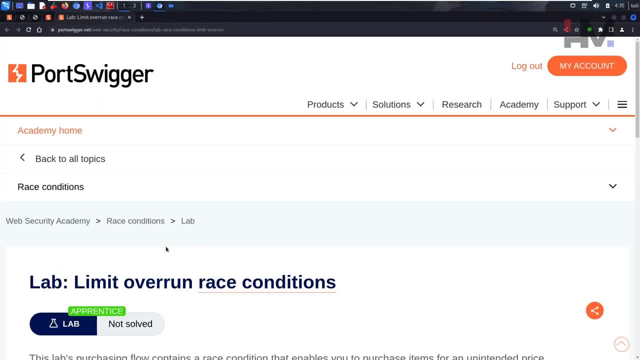 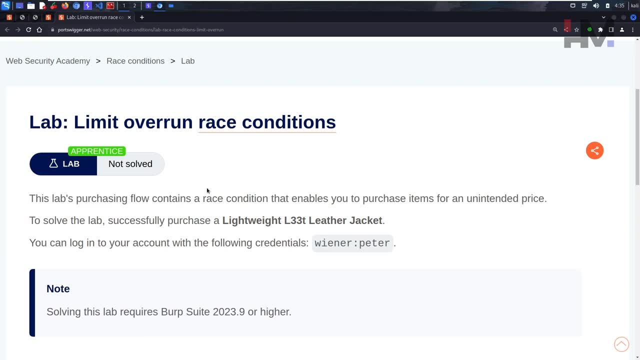 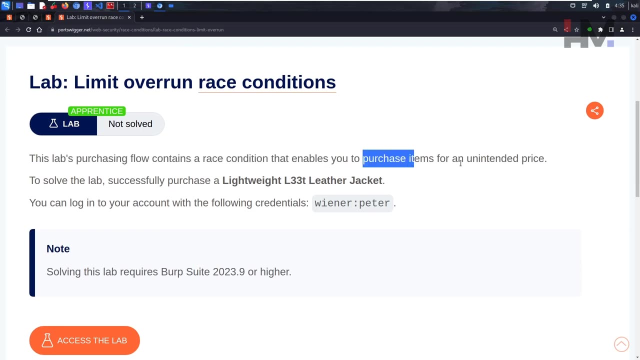 Okay, Let's see a lab, and this is the one. Okay, What does this lab says: Limit overrun, race condition. Okay, So this lab's purchasing flow contains a race condition that enables you to purchase items for unintended price. To solve this lab successfully, purchase a lightweight lead leather jacket. 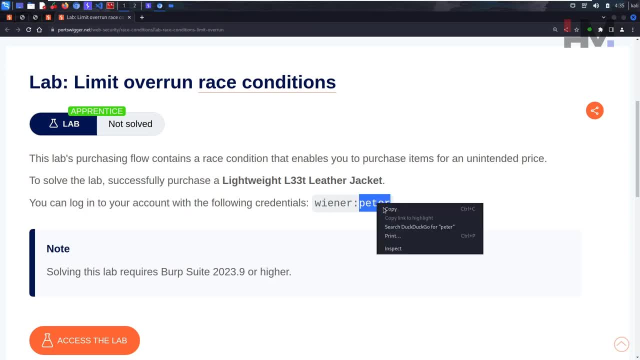 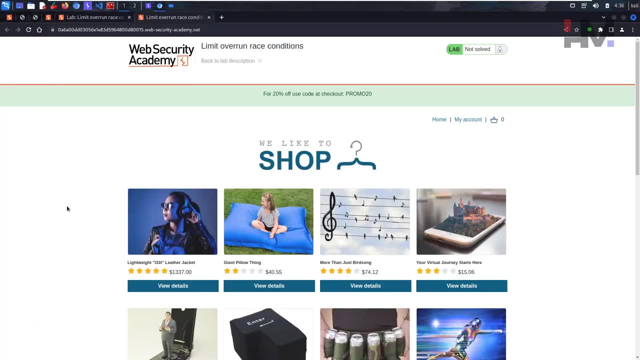 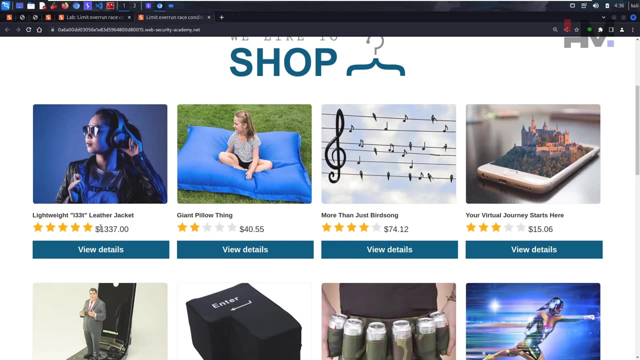 Okay, You can log in using these credentials. Okay, And please make note that solving this lab requires this particular version. Let's access the lab. Okay, So this is the lightweight lead leather jacket. Right, So this is too costly. Let's see how much we have in our account. 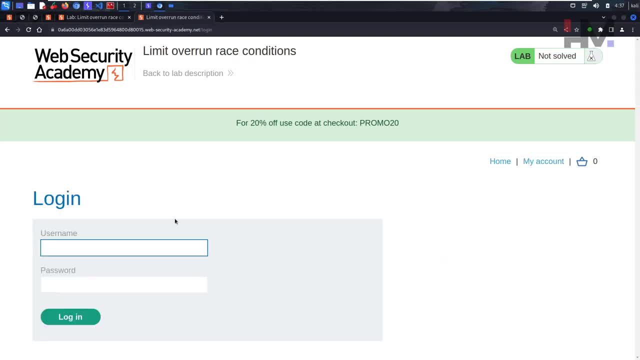 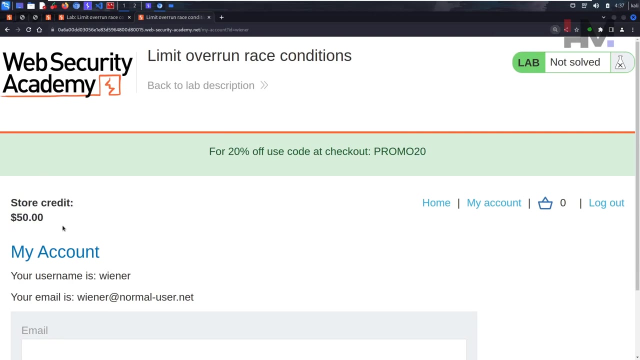 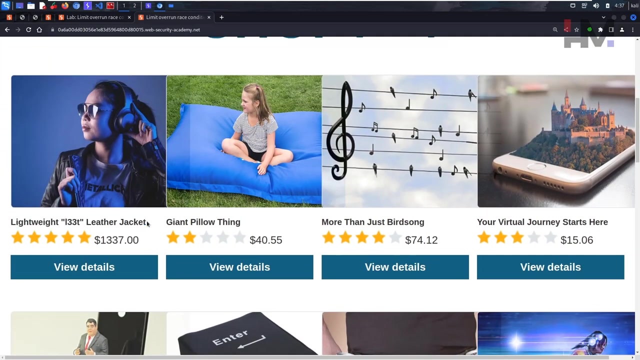 Okay, So let's click on my account. Okay, It is not logged in, So let's use these credentials. Okay, Weiner, Peter, We have a store credit of $50.. So let's go back to home. Let's scroll down and this is the lightweight lead leather jacket. 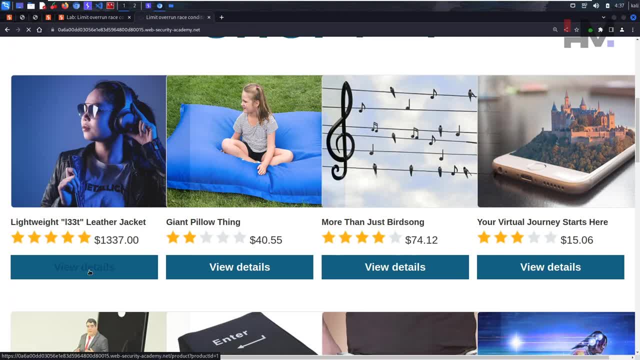 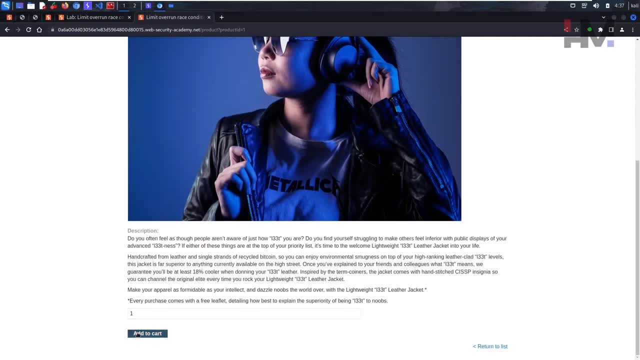 Right, So let's view details and let's scroll down. So it is saying add to cart. As you can see, we don't have anything in the cart, Okay, So if I click this, one product is being added here. Okay. 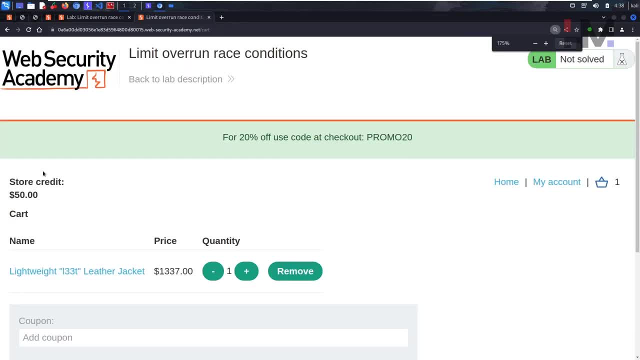 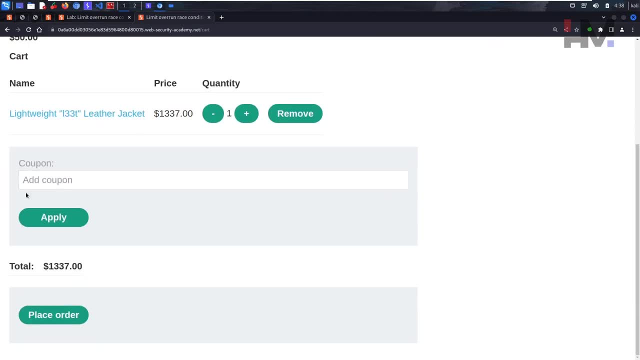 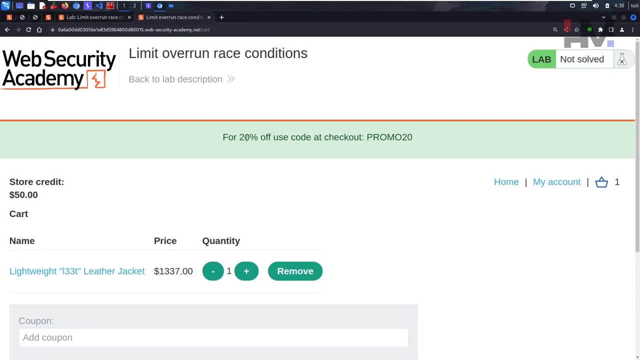 So if I click this one so we are redirected to this particular cart. Okay, We have our product here which is this much costly. They have an option to keep a coupon here. Okay, So do we have a coupon? and at the top we have a promo coupon. 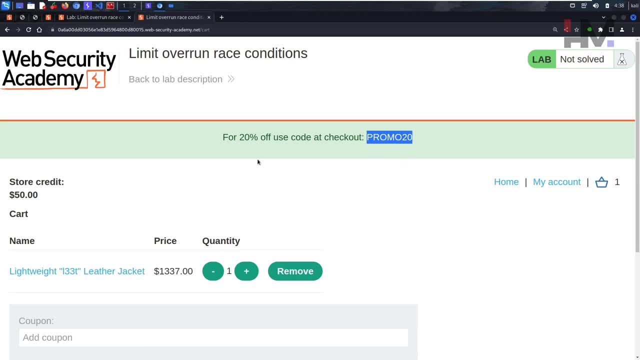 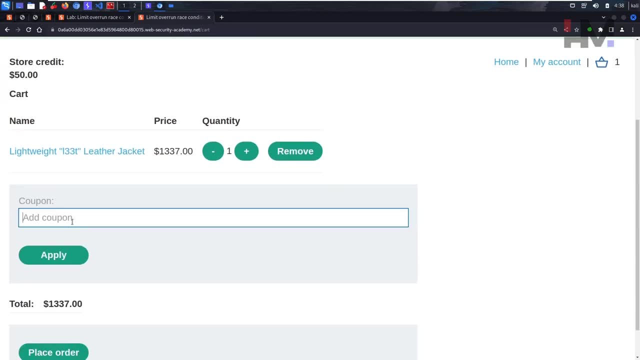 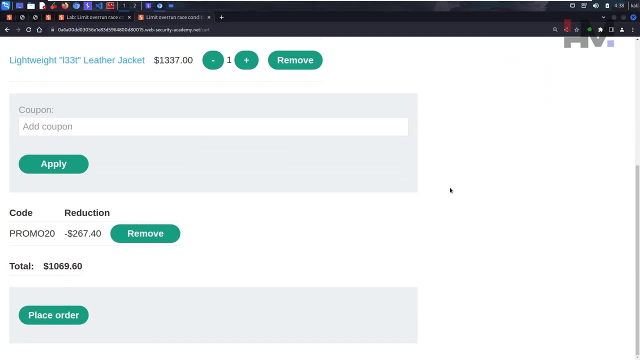 Okay, So promo 20 will reduce 20% of this price. Okay, So that's what they are saying. Let's try to apply this. promo 20 apply, And if I scroll down, I can see that this much is being reduced. 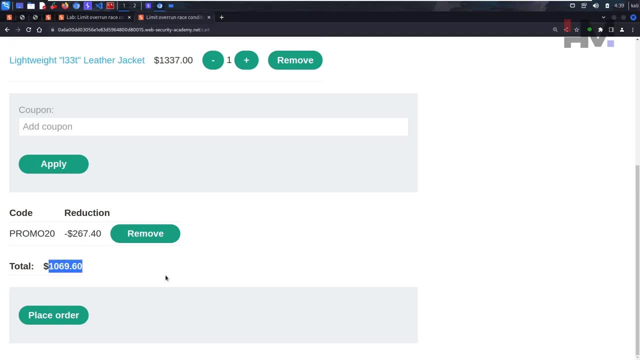 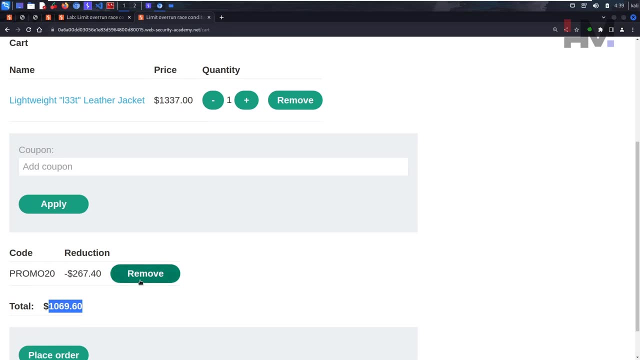 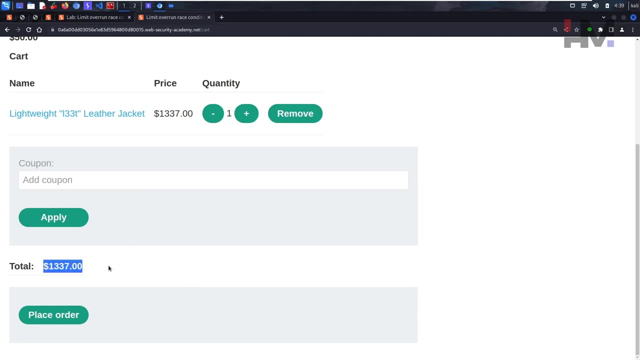 Okay, So this is the total amount that I have to pay now. Okay, So the option they have given is I can remove this particular coupon code. Okay, So, let's click on this remove. Okay, So the total is now. change it back to 1337.. 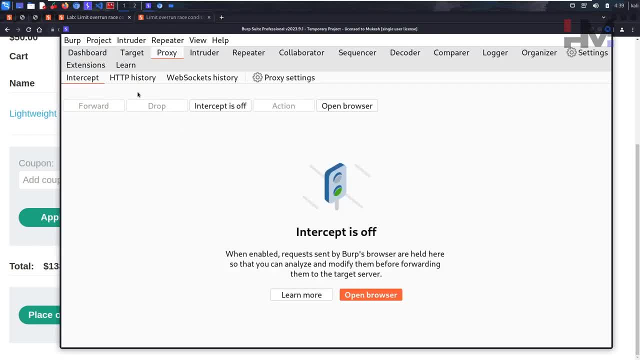 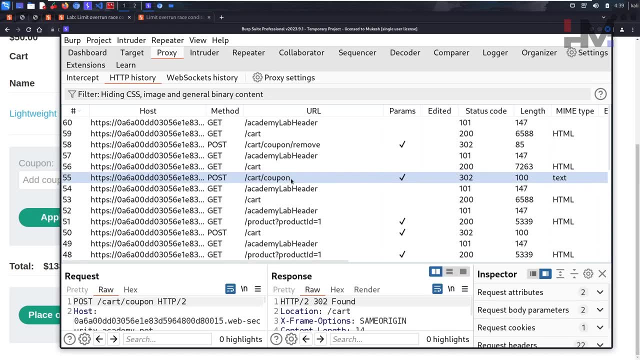 Let's go back to burp suite. Okay, Let's click on history. As you can see, here we have slash card slash coupon And here we have slash card slash coupon, slash remove. This seems to be the request that has applied the promo code. 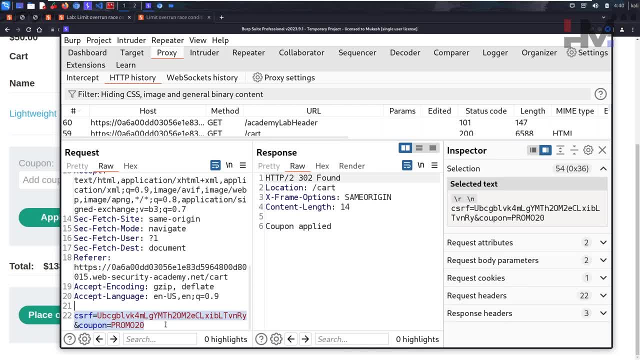 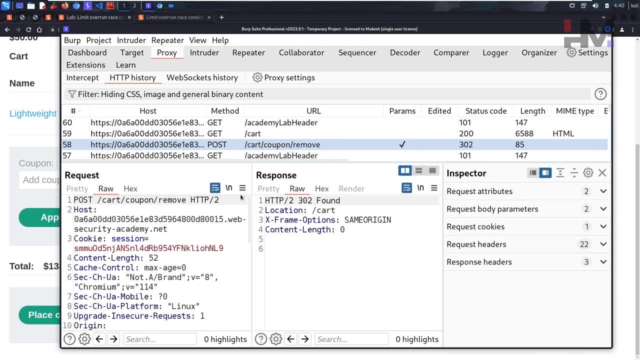 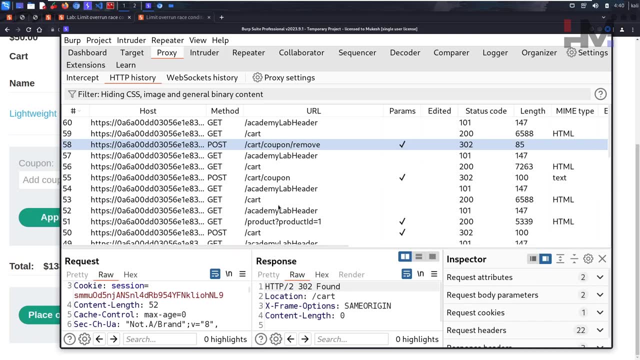 Okay, So, as you can see here, this is the promo code that is being applied. Okay, So, this is the coupon code that is being removed. Okay, So, this being removed, right, So what we are doing is we have to take this particular request, okay, in which we are. 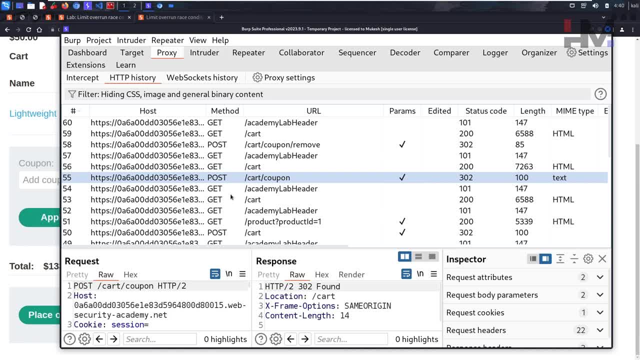 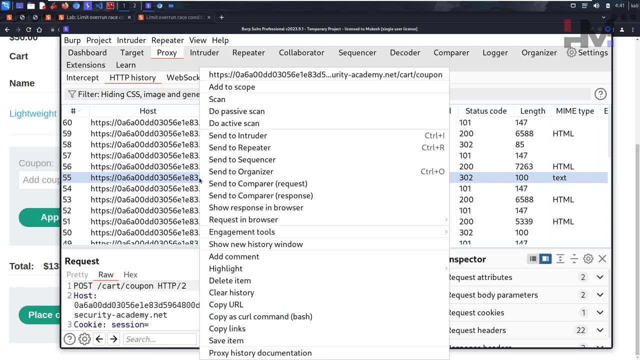 applying the promo code and we have to apply it multiple times parallelly at the same time. Okay, Let's send this particular thing to repeater. Okay, Let's right click on this. send to repeater. Click on repeater. 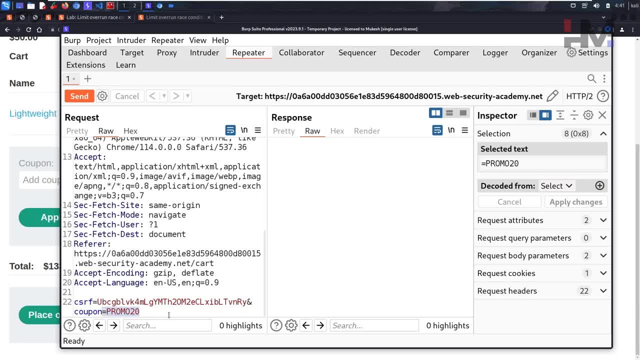 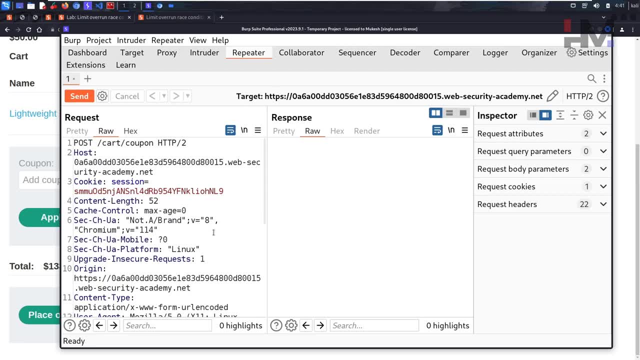 Okay, If I scroll down, I see the promo code. Okay, So if you are upgraded to 2023.9 or higher, then you will see that you will have another option here to create tab group. Okay, This is specifically designed for race conditions. 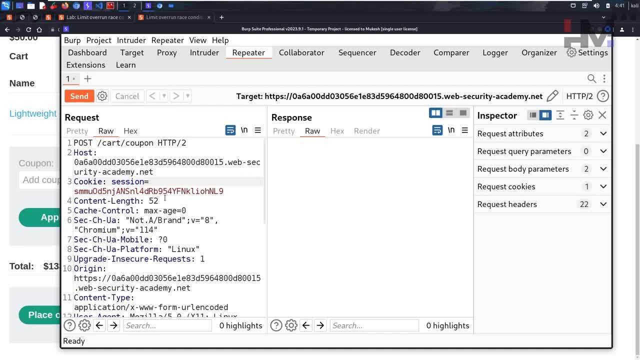 Okay, So in race conditions, what do we do? So we have to send multiple requests at the same time. So in order to send this request multiple times, so you need to create a group of requests. Okay, So how you do is you need to send the same request. 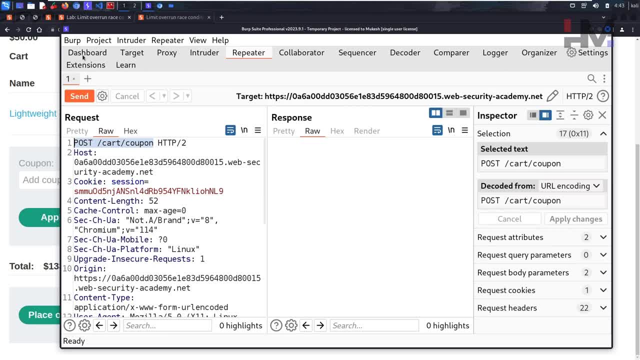 Okay, This particular request multiple times to the repeater. Okay, So you need to create at least 10 to 15 copies of this one. Okay, So how you do is you right click and you send it to repeater. Okay, 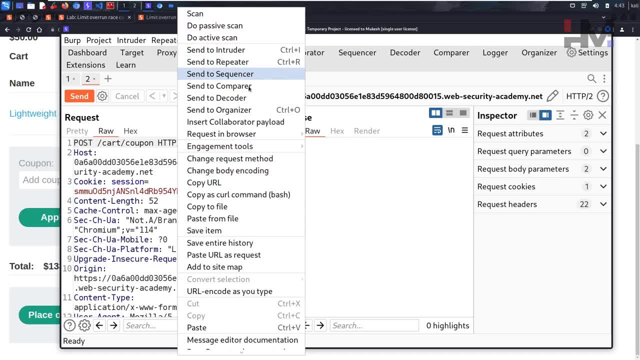 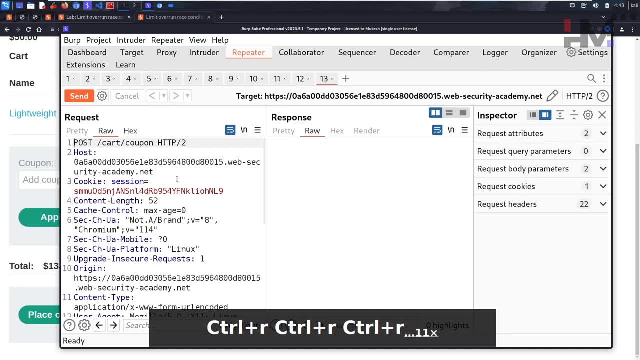 Right click And there is a shortcut here. Okay, Control R. You can directly click Control R. Okay, Multiple times. So it will actually create these many requests. So what you need to do now is you need to group all of these requests. 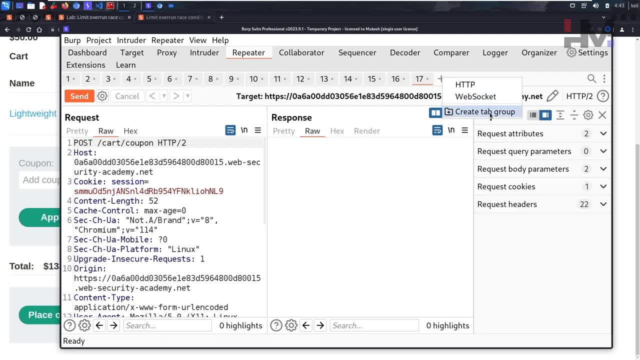 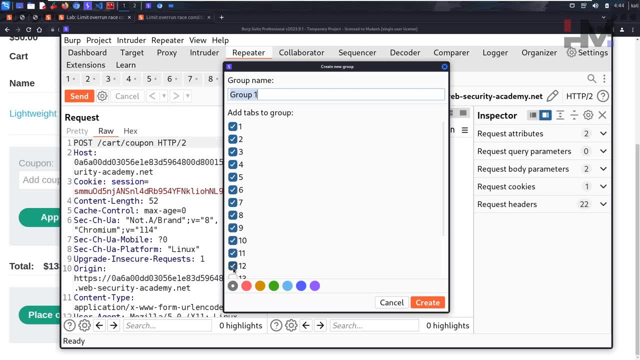 Okay. So how you do that is: click on plus icon, create tab group, select all of them, Okay, And you can give it a name. Okay, This time I'll just give limit overrun, Okay, And you can give any color you want. 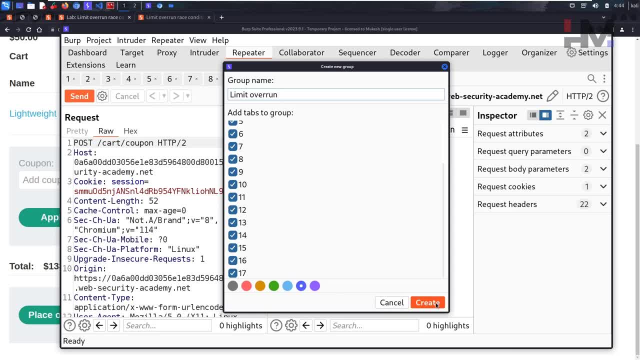 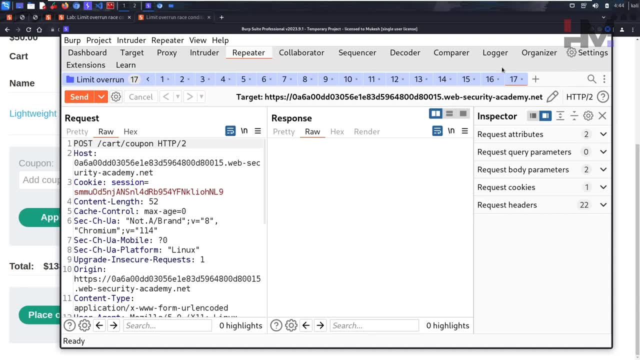 Okay, So I'm just going to give this color and click create. Okay, So this has created a group. Okay, A group of these 17 requests. Okay, You can minimize this using this. Okay, Once you've selected this particular group, you have to send it. 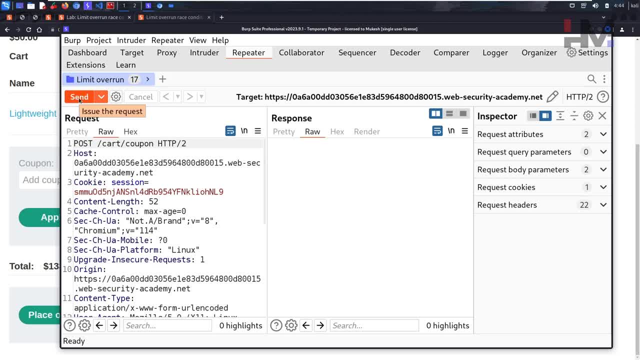 Right, So you should not click this particular thing. Okay, So if you click this, you will be only sending this particular request, So you will not be sending those 17 requests. okay, So you should not click it right away. So what you need to do is you need to change the option. 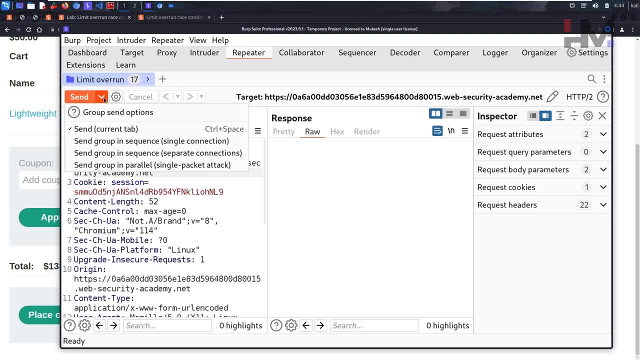 As you can see, there is a drop down button here, So there are multiple ways you can send this. The first one says send group in sequence. okay, If you send a group in sequence, so that is not some kind of race condition, okay. 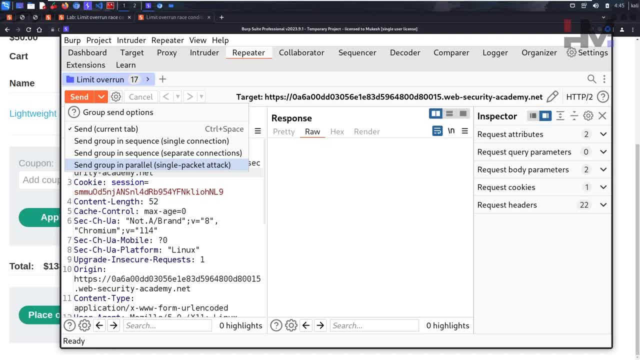 So you have to send a group in parallel, okay. So this is what you need to do: You have to send all of them parallelly at the same time. You need to click on this, okay, And then you need to send this, okay. 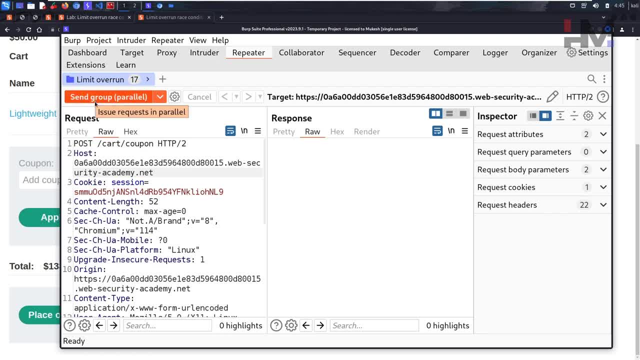 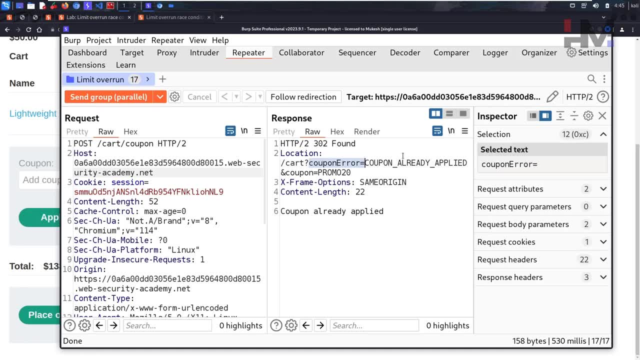 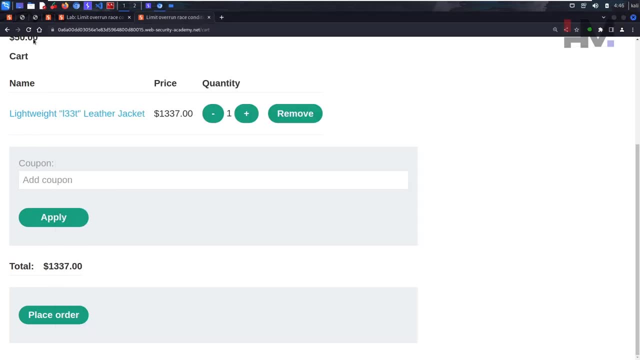 You need to click this again. So when you click this, let's see what's going to happen. As you can see, one of them says coupon code error. Coupon already applied- okay. So let's see What happened here. okay. 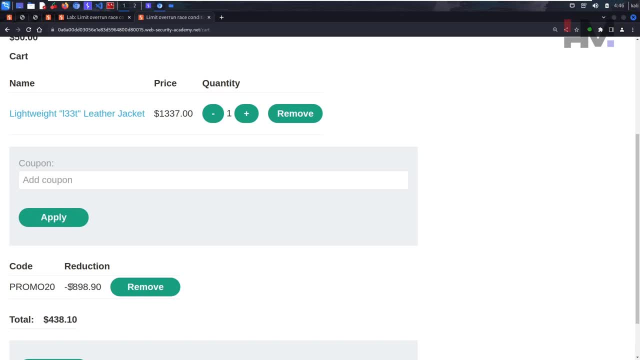 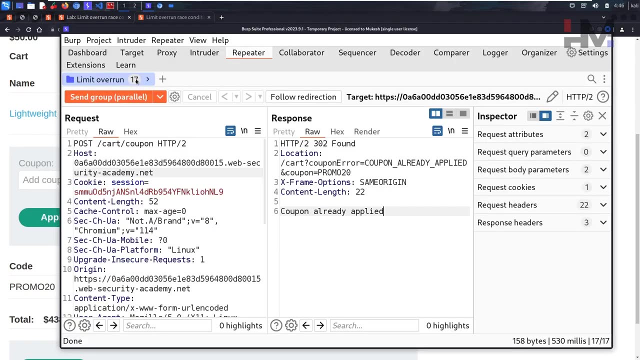 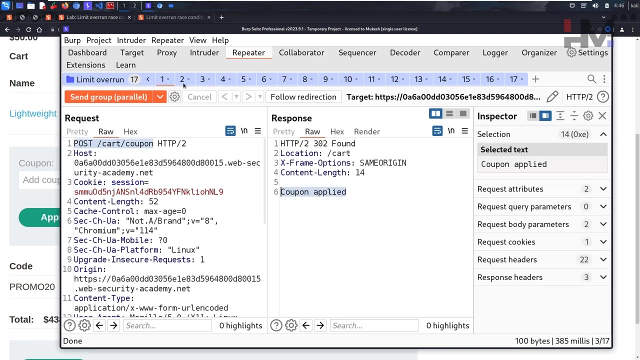 Let's reload this. As you can see, this time we have $899.9,. okay, So this much dollars has been reduced. They have to be reduced because some of these requests had applied this coupon code. okay, Okay, applied coupon code. applied coupon code. 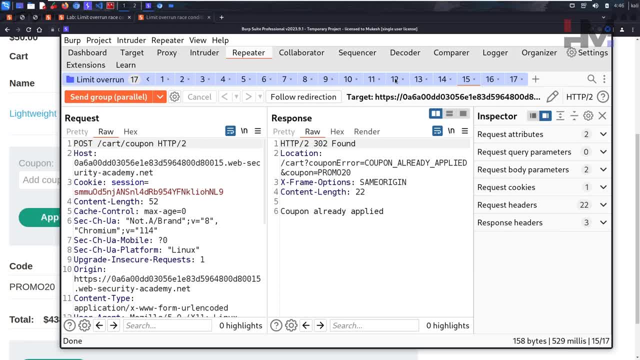 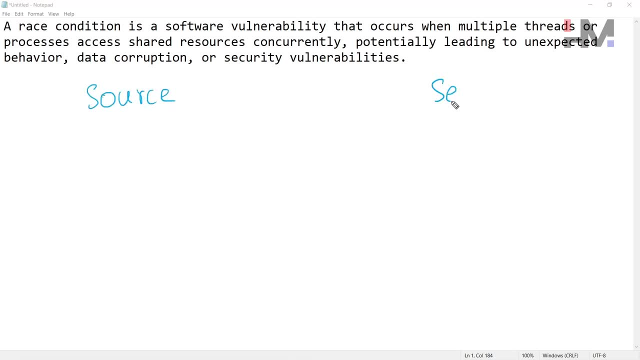 So what is happening here? So it is not sending all the requests in sequence. So they are already sent as a group. Okay, So they are sent in parallel. To explain this, I'll just draw. okay, Let's say this is the source and this is the server. okay, 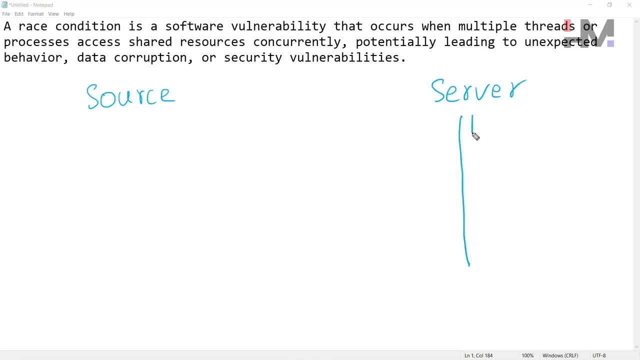 So this has to reach within that window. okay, There is a small gap, okay, Time gap. So this is the race window, okay, So this is where we need to Send out all the requests in this particular location. So when sending a group in parallel, this is not like a single machine gun that is shooting. 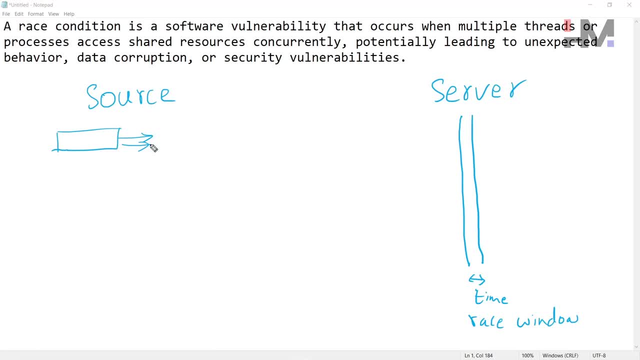 all of the bullets. okay, So it is not like that. So it is like 16 or 17 guns shooting at the same time. okay, So it should be something like this: okay, All of them has to reach within this particular location. 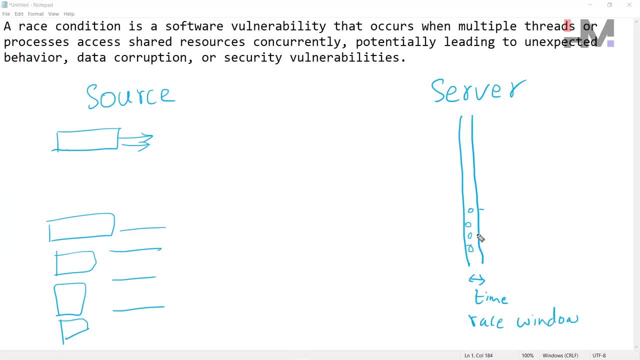 And once these are processed, okay, So we will get some output, So the maximum output that we can get using as many requests as possible. okay, So this is not a single thing that is doing. These are like multiple requests at the same time. 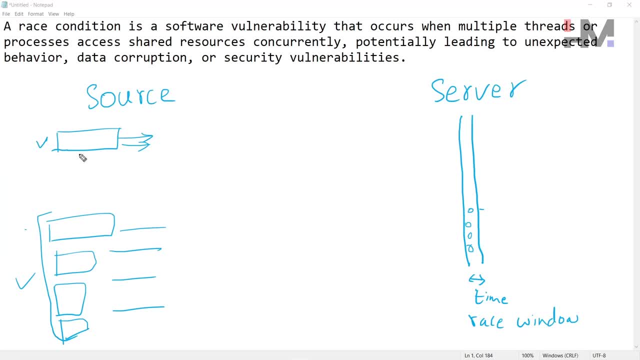 These are like 17 machine guns shooting one bullet. This is not like one machine gun shooting 17 bullets at the same time. okay, This is not like this. This is like this. Okay, Let's go back to the lab. So let's try it again. 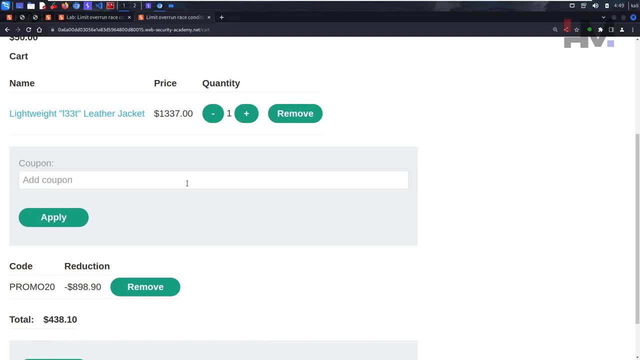 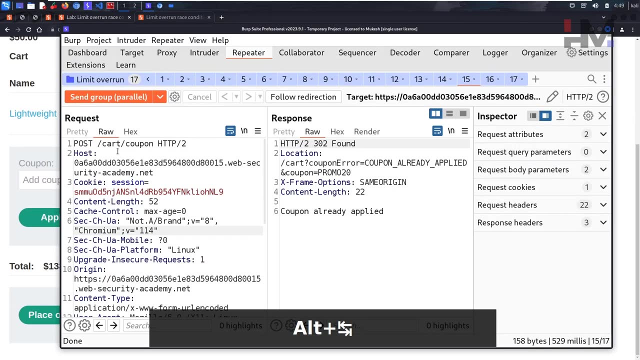 But before trying, so you need to go back to the browser and remove this one. Okay, So remove this. Okay, Now we are back again. So let's apply the same promo code again. So let's reload and see what happened. 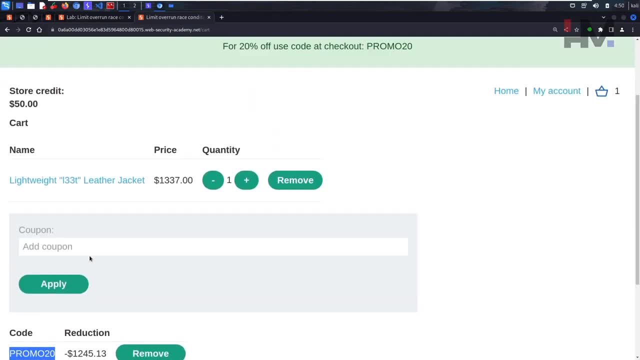 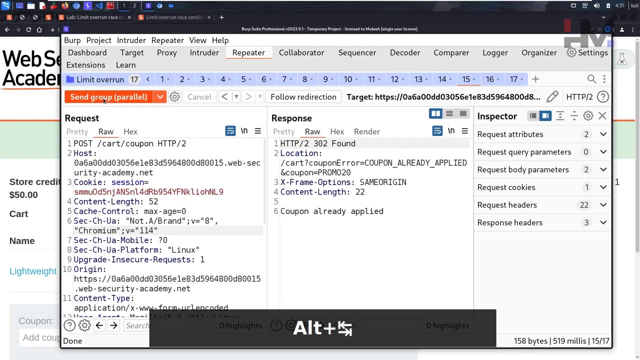 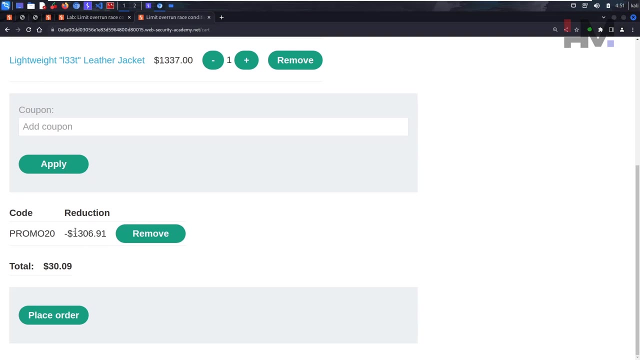 This time it is even less, Since we have only $50, we cannot afford it. Okay, So you need to delete it And you have to send it again. Okay, Send group in parallel. Okay, Reload. All right, As you can see, this time $1,300 has been reduced, okay.